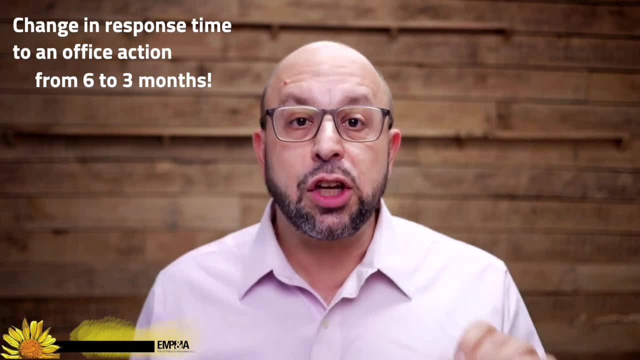 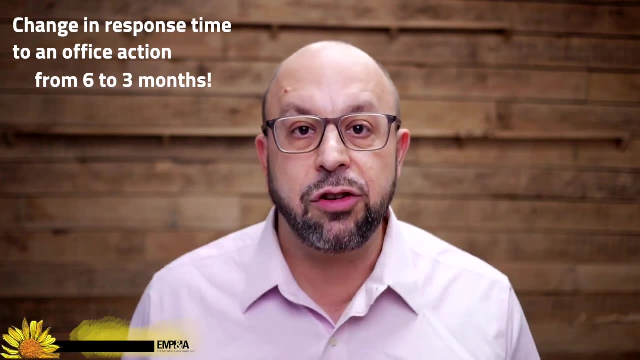 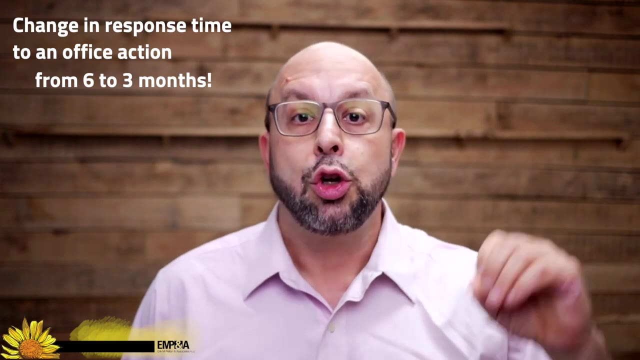 cutting the time period in half. This is a huge change, especially for law firms and the way they manage their caseload. It's also going to be a change for client communications and for clients to have to make decisions and provide information to their counsel to help with a 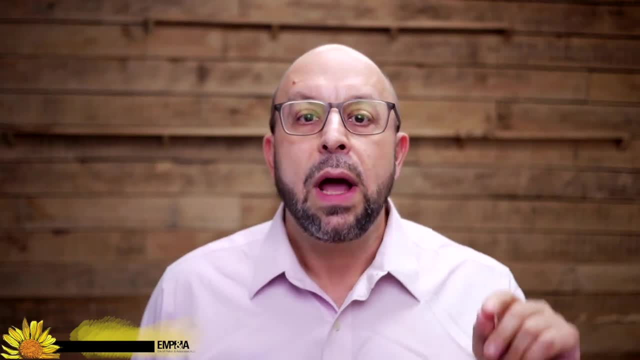 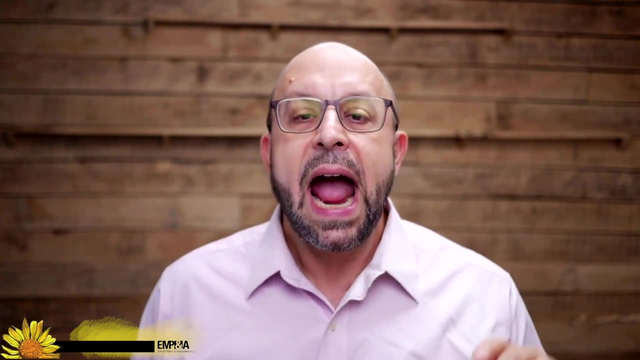 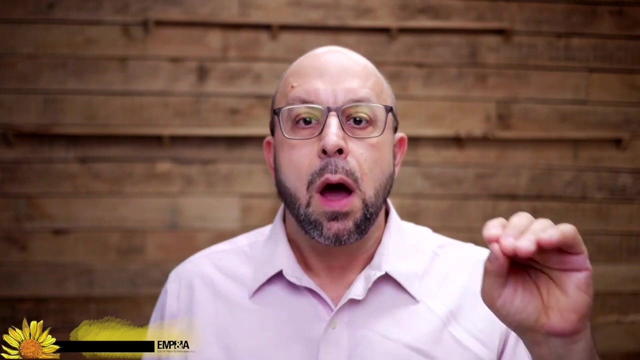 response. So the USPTO is changing the time period for most applicants to respond to an office action. Now it doesn't impact all applications- Some foreign-filed applications will not be subject to this rule- And it doesn't impact office actions issued post-registration, which are relatively 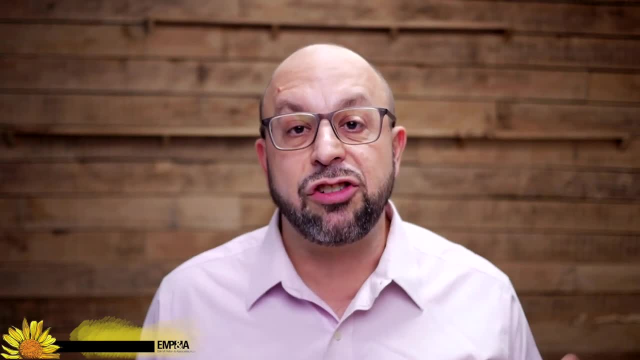 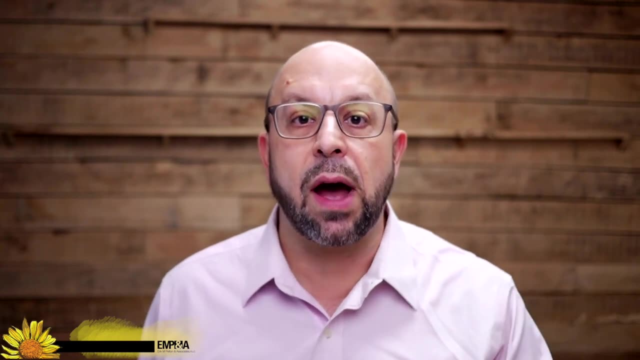 few and far between, And so when we talk about an office action generally, we're talking about a pending application, And all pending applications, except for some of those foreign-filed ones, will not be subject to this rule. So the USPTO is changing the time period in half. 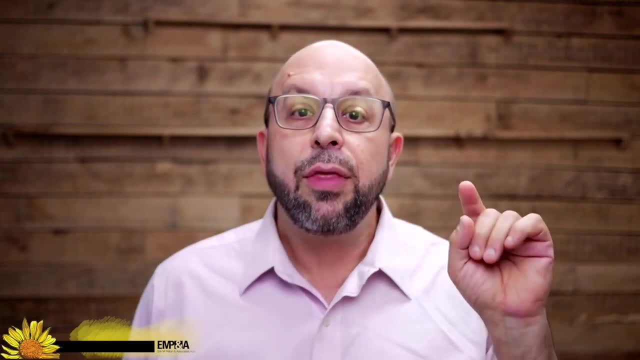 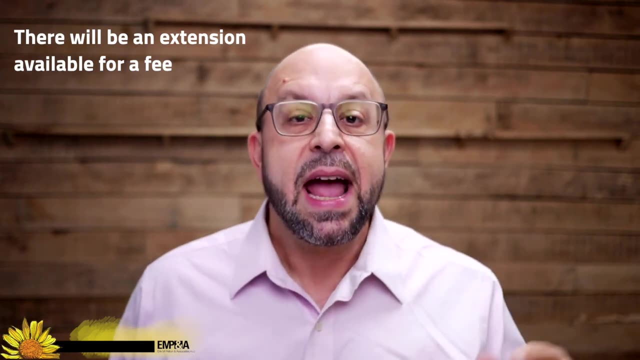 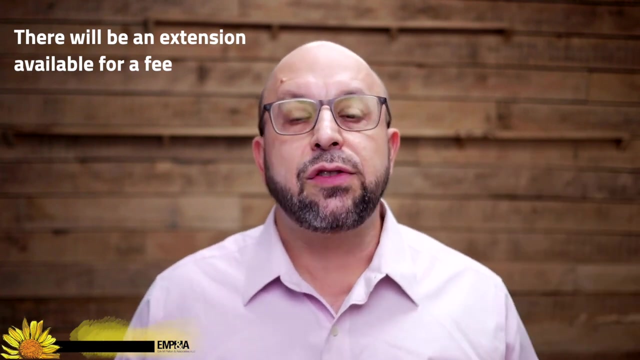 The USPTO will now have a three-month response deadline. There will be an extension available for a fee, but that's an additional fee And that's an additional deadline to keep track of and a filing to submit. And so, while it's good that there's an extension available, 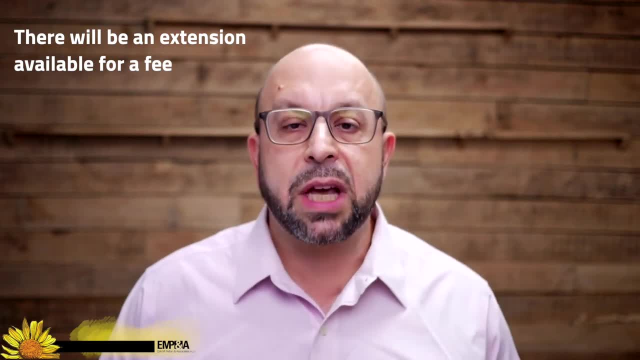 it's not the same as what the current system is, because there's more work that goes into getting an extension and more costs, And so the USPTO is changing the time period in half, And so, while it's good that there's an extension available, it's not the same as what the current 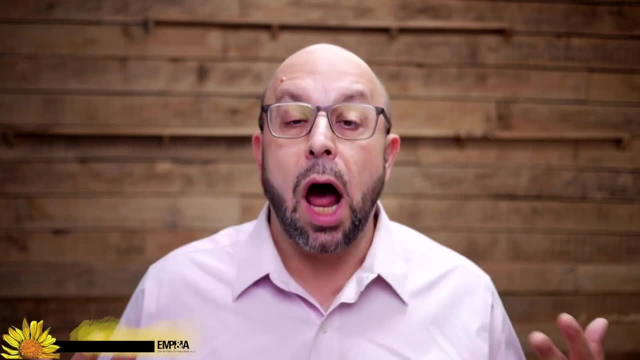 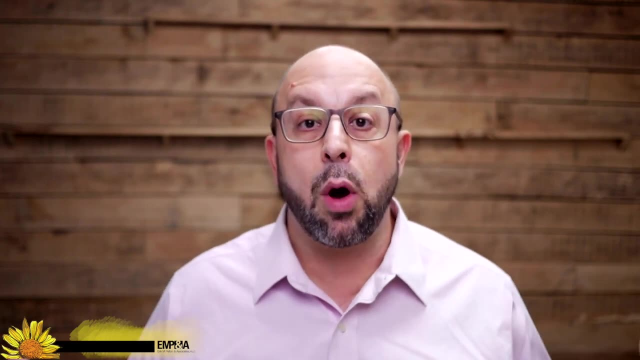 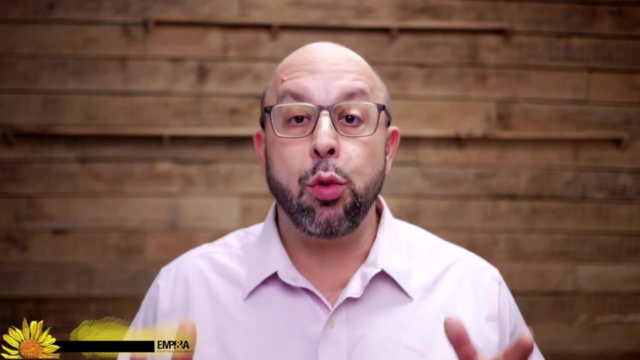 system is because there's more work that goes into getting an extension and more costs. So I am really not pleased with this change. I voiced some of that displeasure when the rules were being proposed. However, it is what it is. The rule is now upon us imminently, And this new 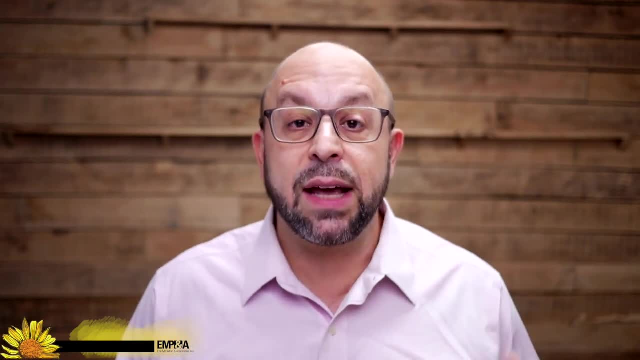 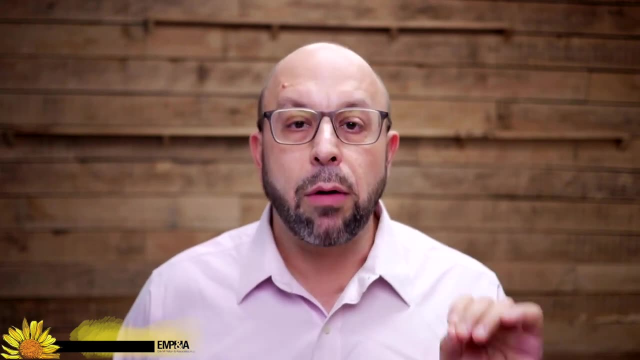 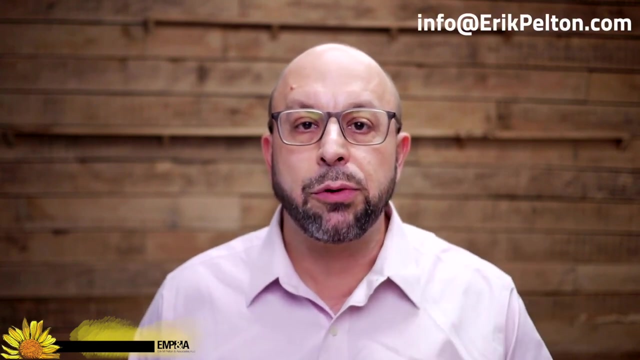 three-month response period is the biggest change that I have seen to trademark practice in many, many years. If you have questions about the new rule or about other trademark issues, feel free to reach out to me. info at erikpeltoncom, That's E-R-I-K-P-E-L-T-O-Ncom. 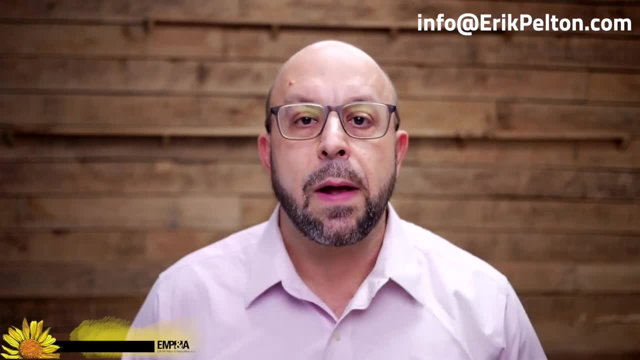 Or visit the website and you can find a Connect With Us button there.